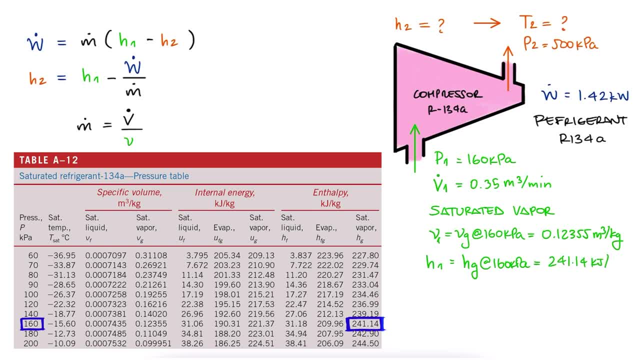 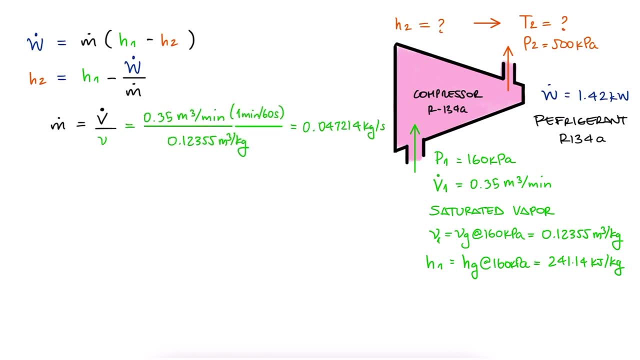 is the specific enthalpy Hg for our enthalpy value at state 1.. With this Vg value and doing a simple unit conversion, we find the mass flow rate. We substitute the mass flow rate, the specific enthalpy at 1 that we just wrote down and 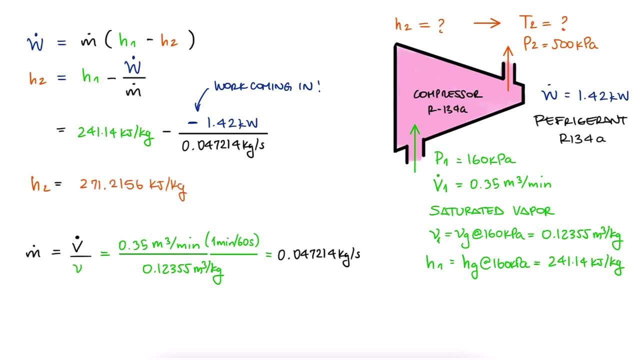 the power to calculate the specific enthalpy at state 2.. Now that we have the specific enthalpy and since we're given the pressure for state 2, we look up superheated tables for R134a specifically for that pressure and find the temperature. 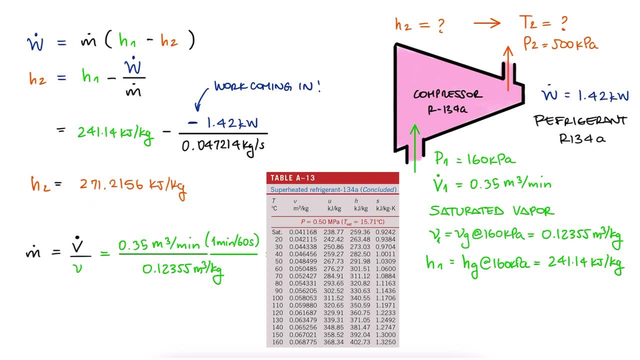 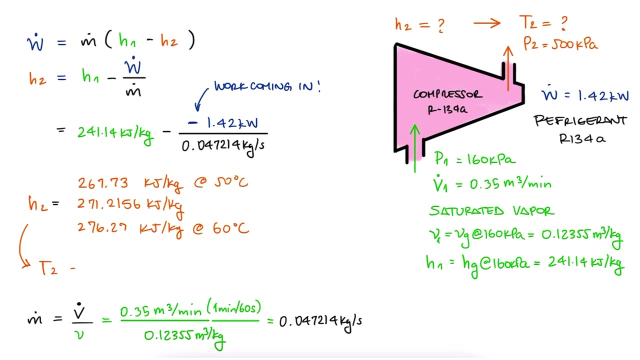 that corresponds to that specific enthalpy value. To do this we need to interpolate. We see that 271 is between 267.73 and 276.27, which correspond to 50 and 60 degrees Celsius. We do a simple interpolation and check the interpolation examples linked below, if you. 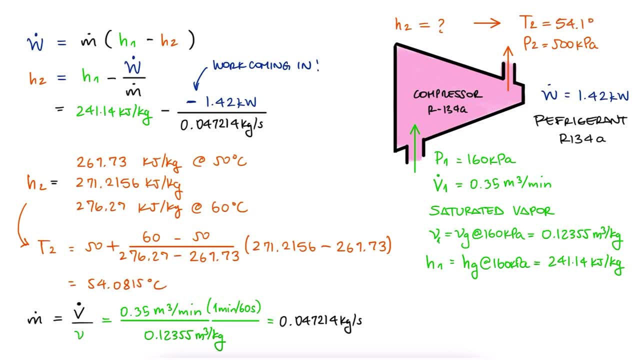 forgot how to do this and find that the temperature is 54 degrees Celsius. If you want to check out other examples in the turbines, compressors and pumps topic, make sure to check out the links I left down in the description below. 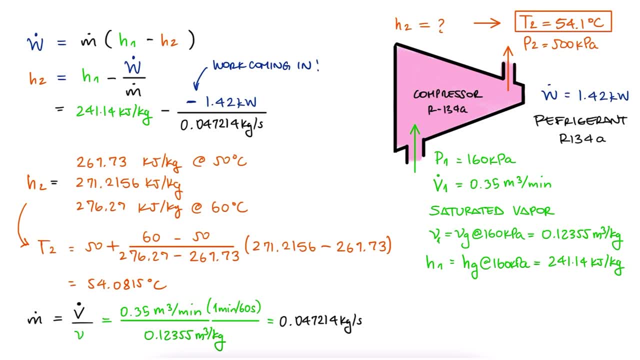 You'll find the links to the other lectures of the thermal course, as well as other engineering courses. Thanks for watching. 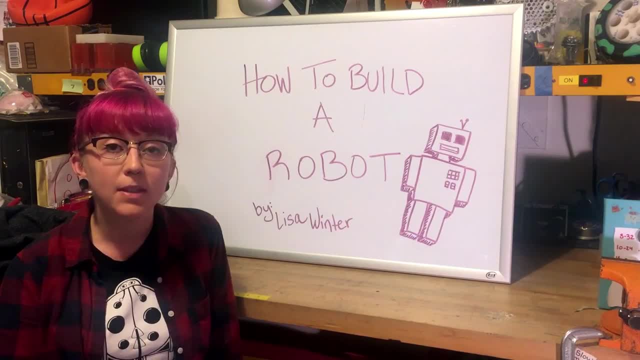 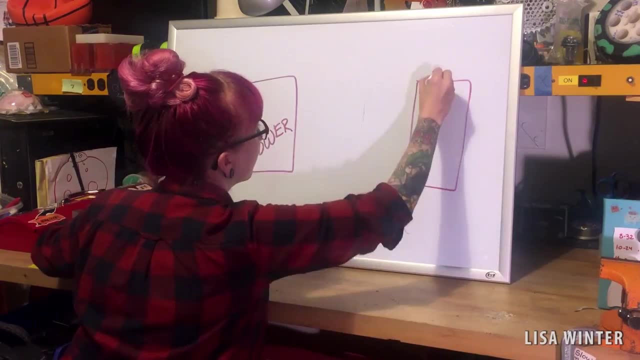 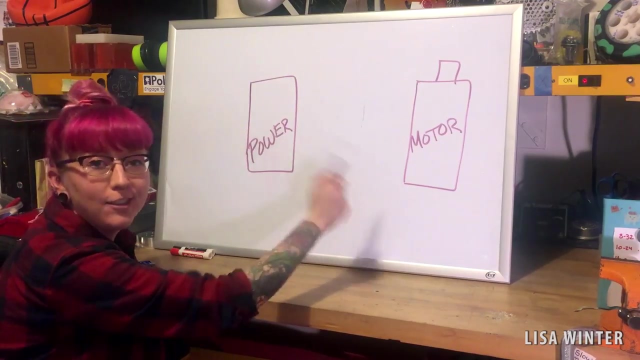 Hi, in this video I'm going to teach you how to build a robot. It may sound hard, but the concept is really quite simple: How to build a robot, Robot, Robot. First, you have your power and your motor, and you want to put the power into the motor to make it run. 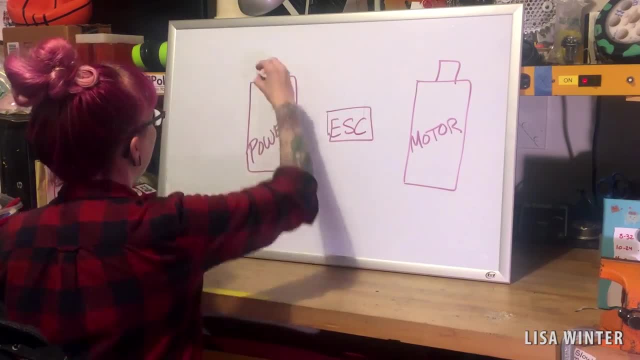 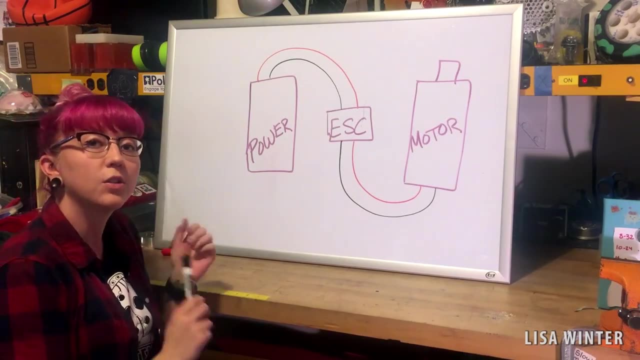 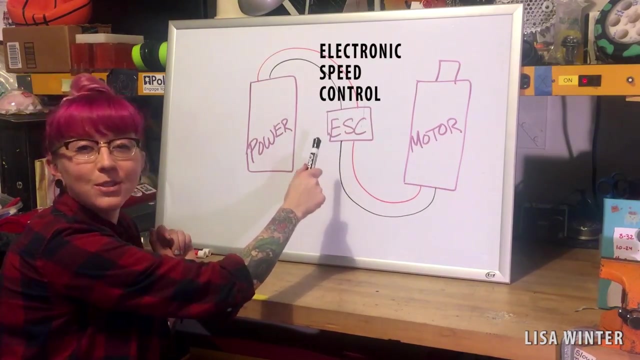 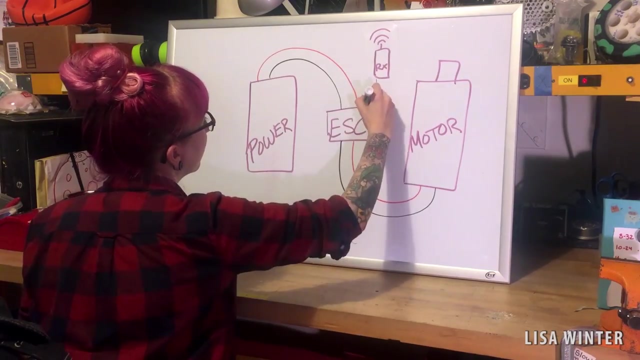 In order to control how much power you put into your motor, you need a speed control, and this literally controls the speed. The next action is to add a receiver and the receiver is going to be a speed controller. The next action is to add a receiver and the receiver is going to be a speed controller.